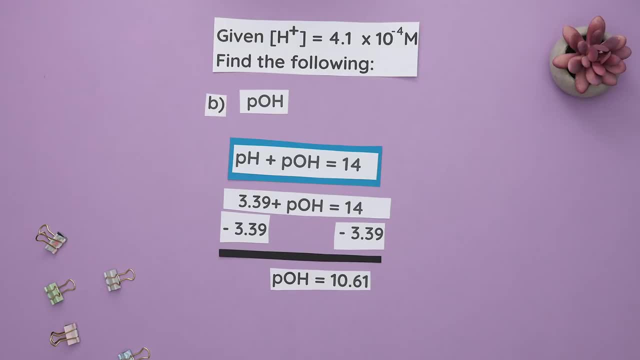 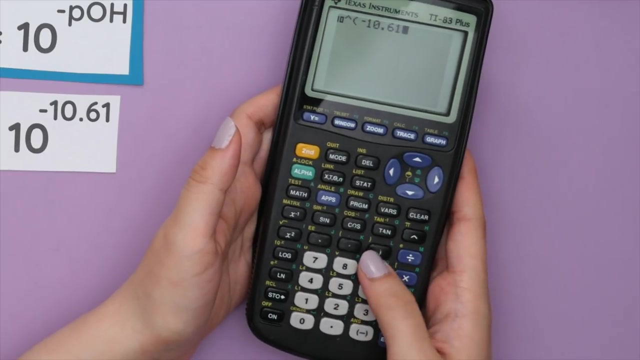 Since we just found pOH and we are now finding the concentration of base, we can use this formula and plug in the pOH. Plugging this into your calculator, make sure to press 2nd log and then put the exponent of negative 10.61.. 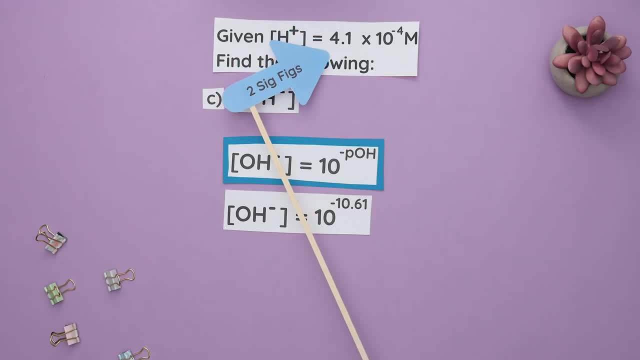 Round two sig figs, since our initial acid concentration had only two sig figs. This gives us 2.5 times 10 to the negative 11th and our units are in molarity, since concentration is measured in molarity. In question two, we are given the pH and asked to find our acid and base concentrations and the pOH. 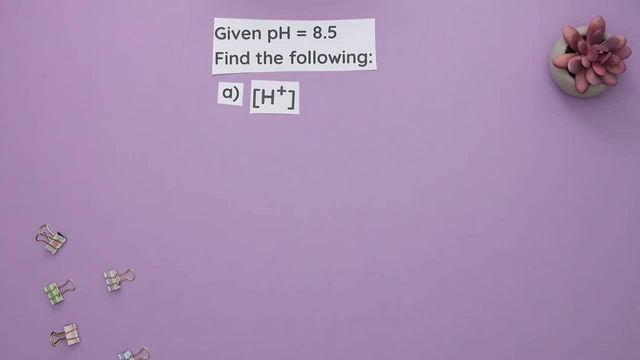 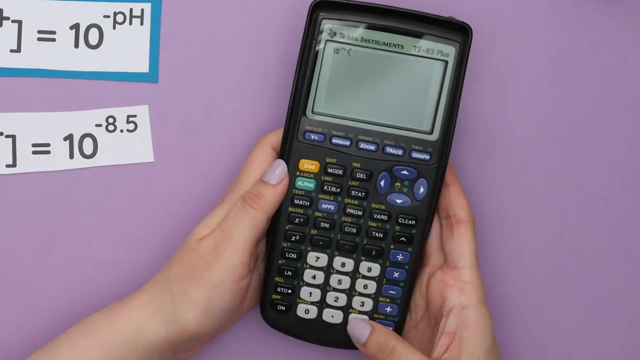 Starting with part A, we are given the pH. We can use this formula and solve for the acid concentration. So press 2nd log on your calculator, then input the exponent of negative 8.5 and we get this as our acid concentration. 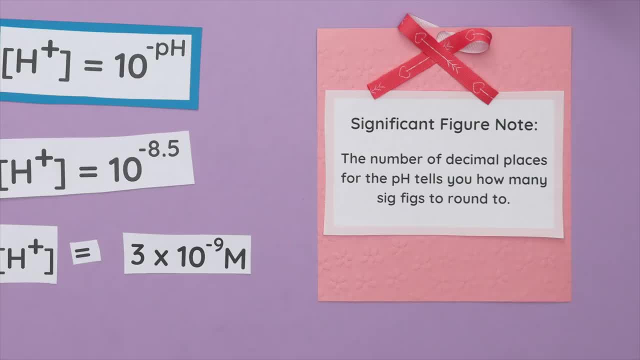 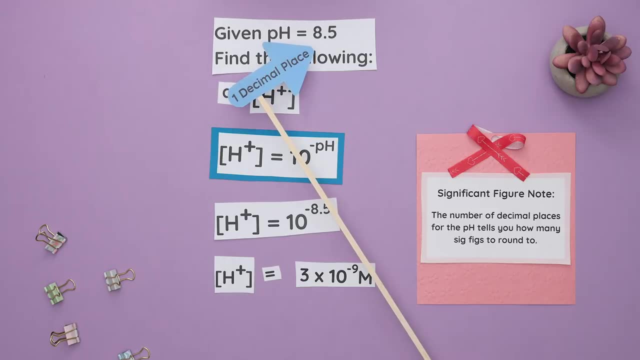 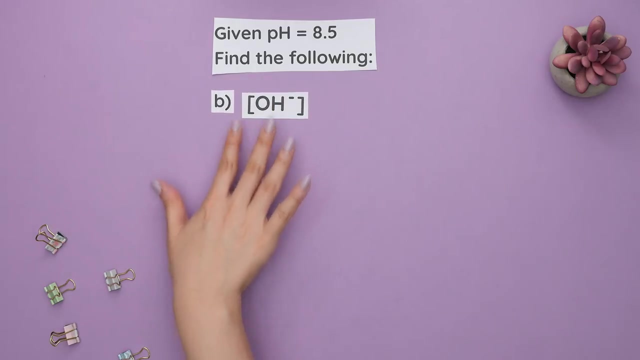 Significant figure note when we are going from pH to acid concentration. the number of decimal places for the pH tells you how many sig figs to round to. This is why our acid concentration only has one sig fig. Part B to find our base concentration. 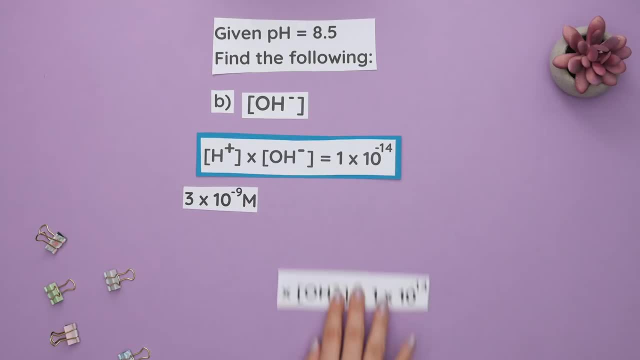 we will use this formula and plug in the acid concentration we just found, Divide both sides and we will get this as our base concentration, rounded to one sig. fig Part C. there are two formulas we can use to find pOH, in this case. 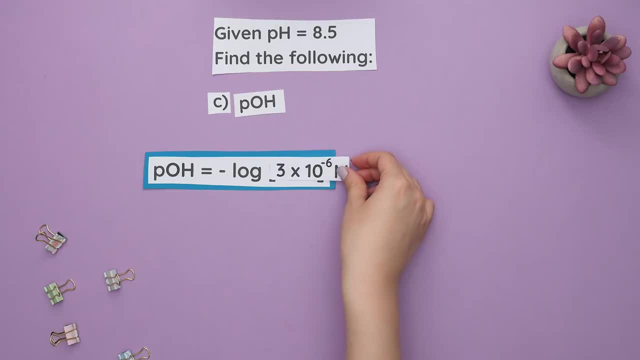 Here's the first formula. We'll plug in the base concentration to get this as our pOH. The second formula we could have used instead was this one, And we can plug in our pH subtract both sides by 8.5,. 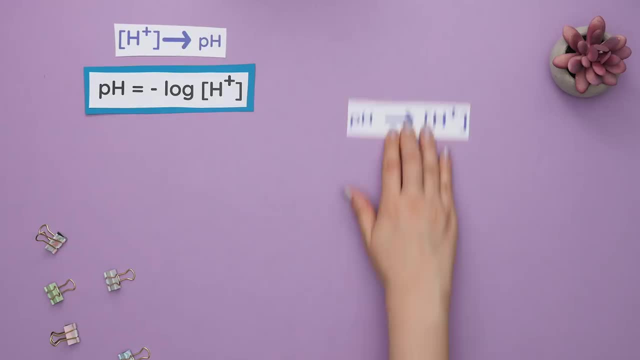 and we would get the same value. Now here's a summary of when to use each formula. When going from your acid concentration to pH, use this formula. Go in the opposite way: from pH to acid concentration. use this Now when you're going from your base concentration to pOH. 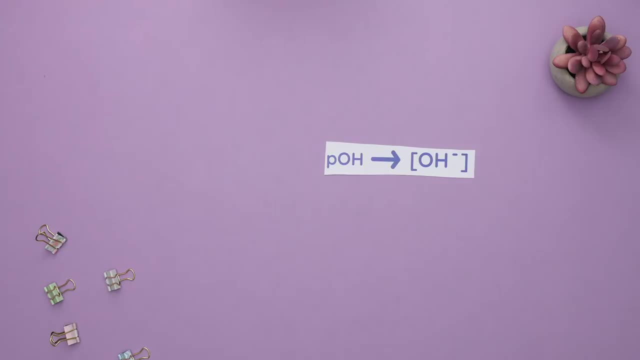 use this formula: Go in the opposite way: from pOH to base concentration. use this If you are given the pH and asked to find pOH, or going from pOH to pH. use this formula Going from acid concentration to your base concentration.